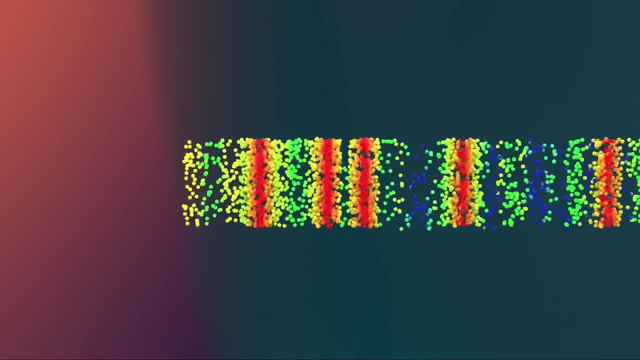 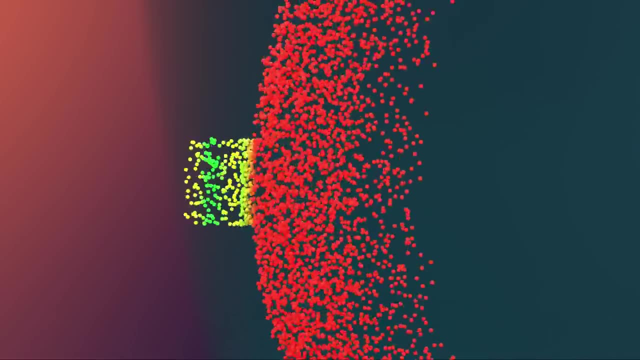 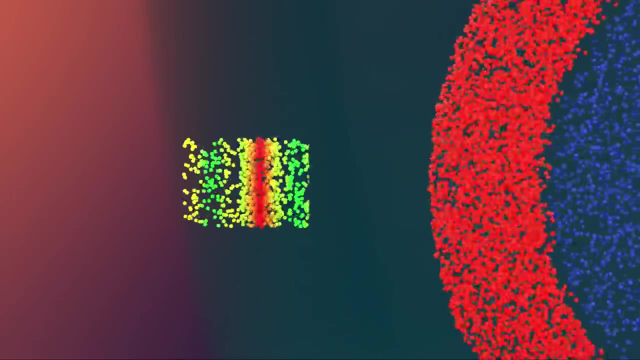 the balloon is popped. You may ask: where does this pattern come from? Well, the high pressure air particles rush out and generate a high pressure wave, But when they do, they create a low pressure void in the balloon's center The air particles rush back in to. 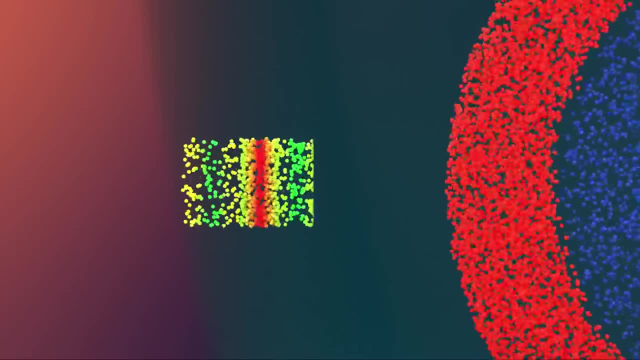 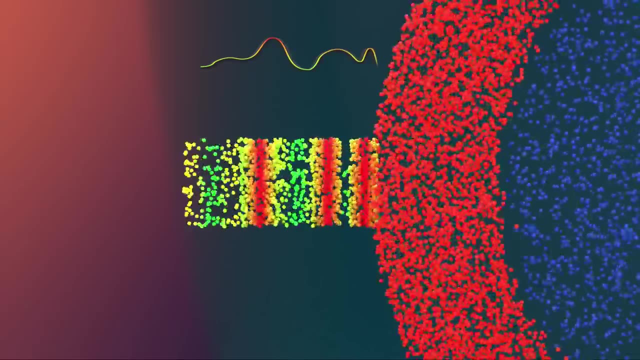 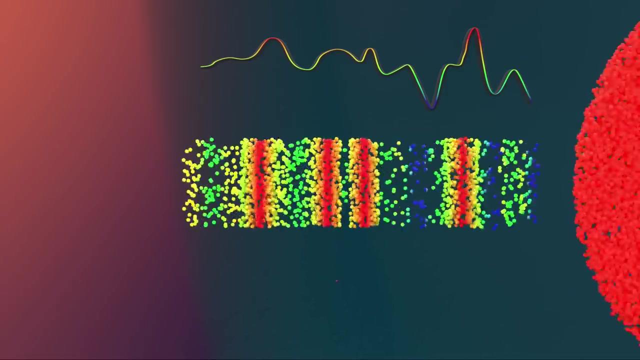 fill this void, thereby generating a low pressure wave. When the particles rush back in to fill this void, they rush in too much, thereby creating a second high pressure zone. This cycle repeats itself, and each time it does, it generates a high pressure and low 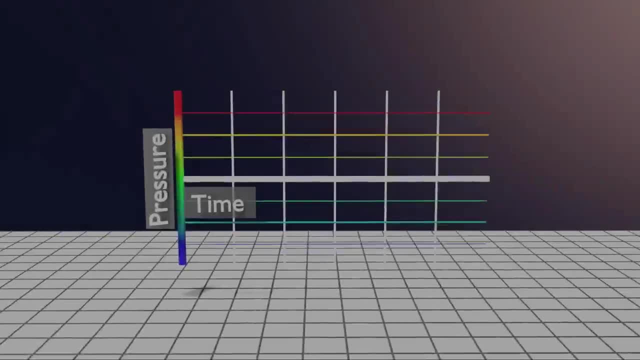 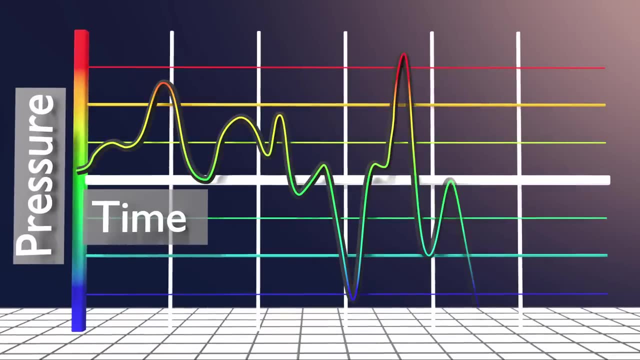 pressure wave, which can be graphed. This graph shows the pressure waves, or waveform produced by popping a balloon. The vertical axis is pressure, or the amount of force the particles bounce into one another. The horizontal axis is time. These high points in the waveform are called compressions, and 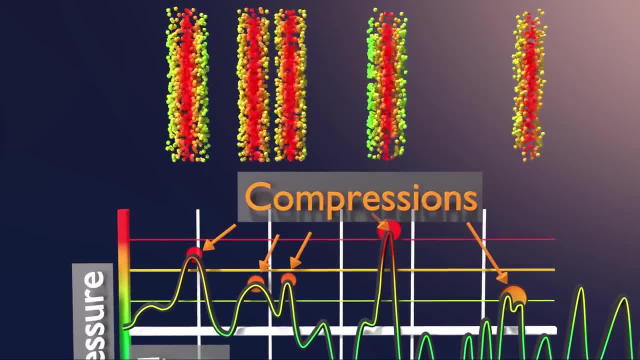 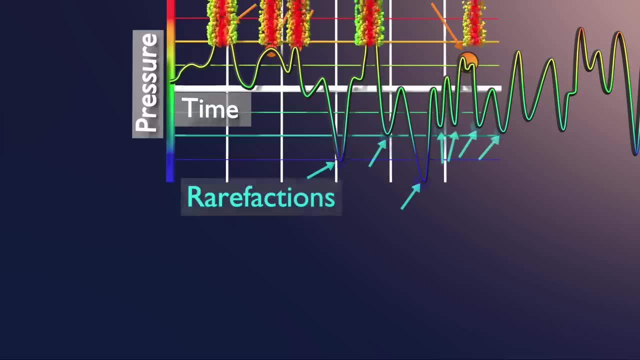 they are where the particles are compressed and bouncing around a lot and thus have a higher pressure. The low points in the waveform are called rarefactions, and they are where the air particles are more spread out and not bouncing around as much and thus have 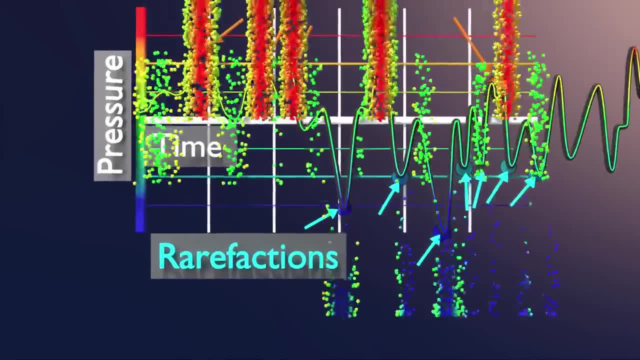 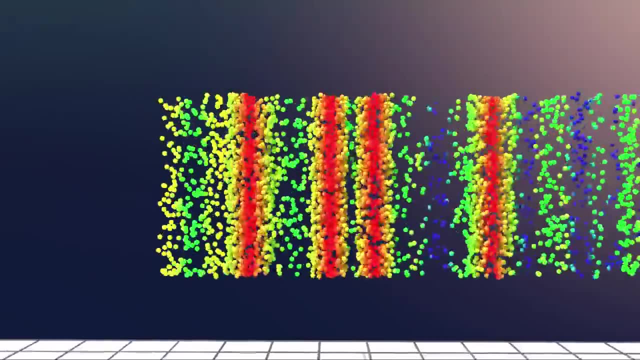 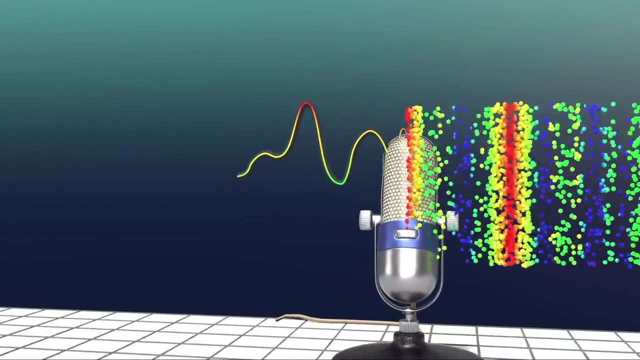 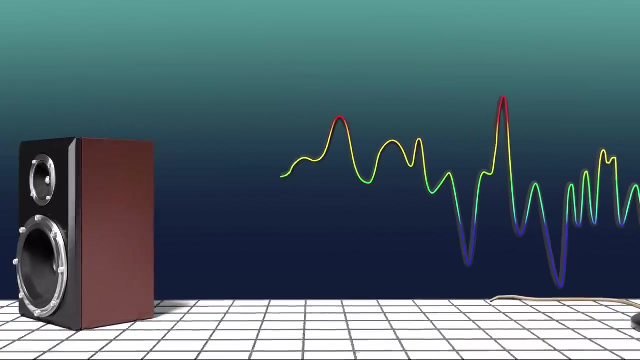 a lower pressure. Both the graph and particle animation help to visualize sound which, as we know, is invisible to our eyes. The measurements are taken at a single point in space. In this case, the pressure was measured by a microphone In order for your speakers to duplicate this sound, the diaphragm in your speakers just. 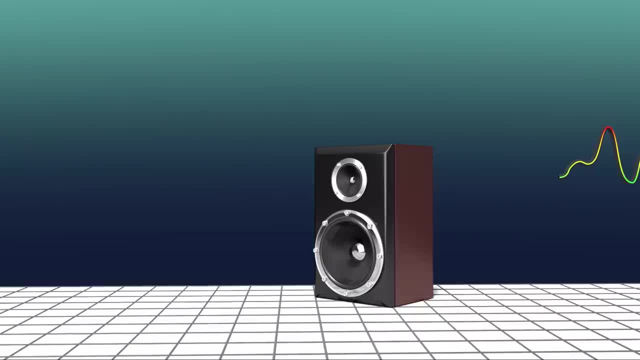 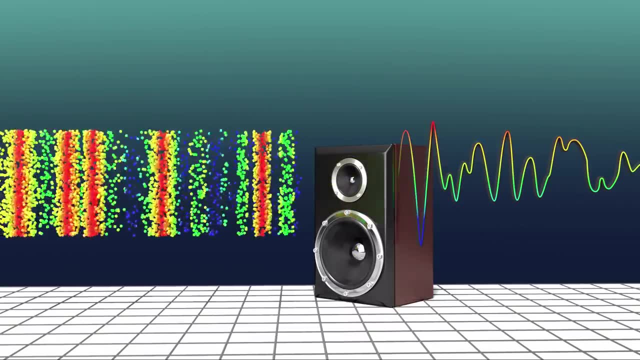 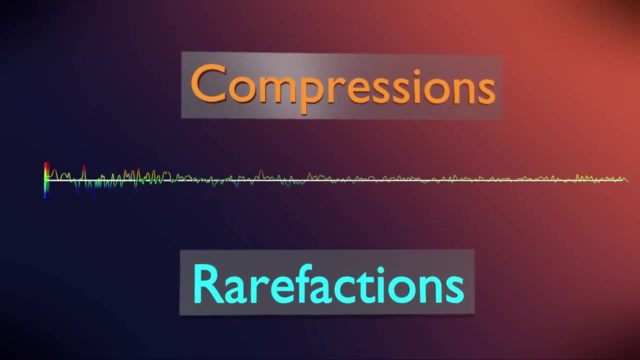 have to move in a similar fashion. The entire sound takes 1 tenth of a second for your speakers to duplicate. This visualization is just the first section of the overall pattern of cycling, compressions and rarefactions produced from a popping balloon In just this quick sound. there were about 50 of these cycles. 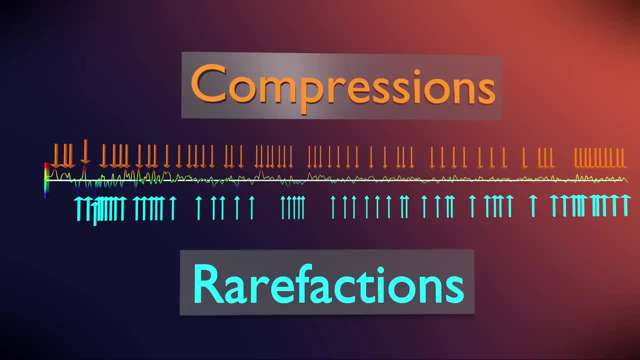 If we slow down this sound to 4 seconds, you can hear some of the cycles between compression and rarefaction. If we slow down this sound to 4 seconds, you can hear some of the cycles between compression and rarefaction. These cycles last much longer than this quick duration. 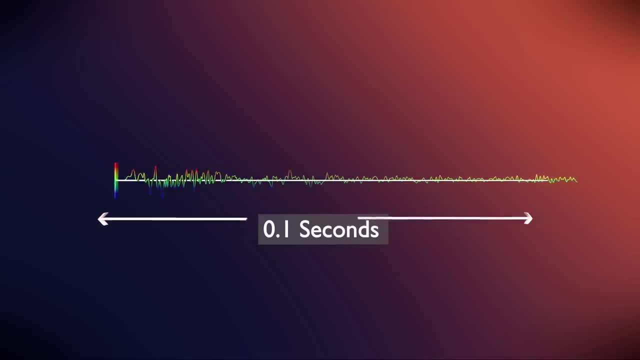 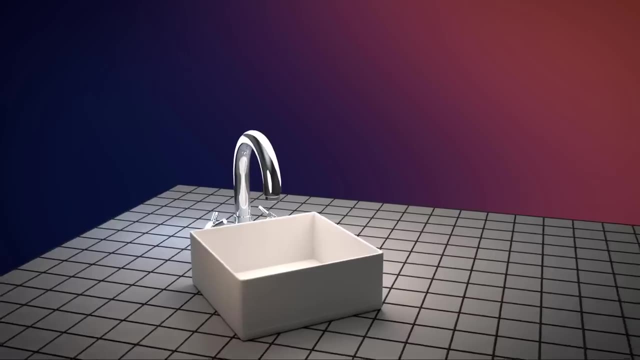 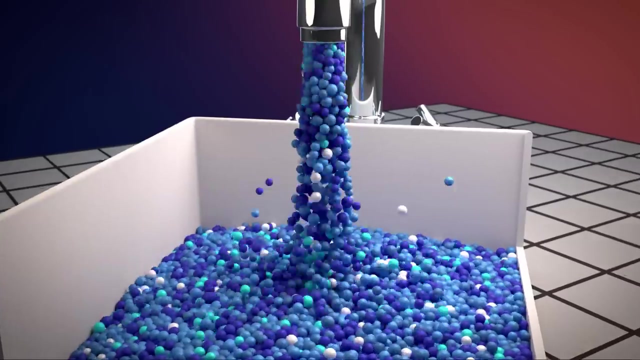 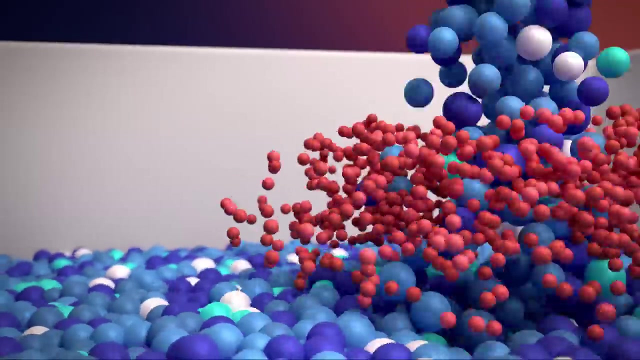 So in visualizations of sounds we usually see the squished version of this graph, which looks like this. Let's consider another sound. Here is a running faucet. The moving water molecules apply a force to the nearby air particles, thereby causing the. 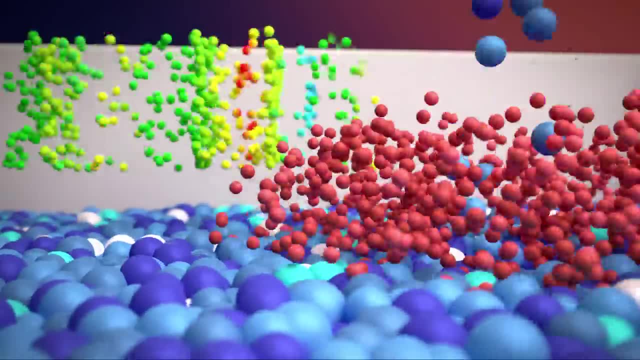 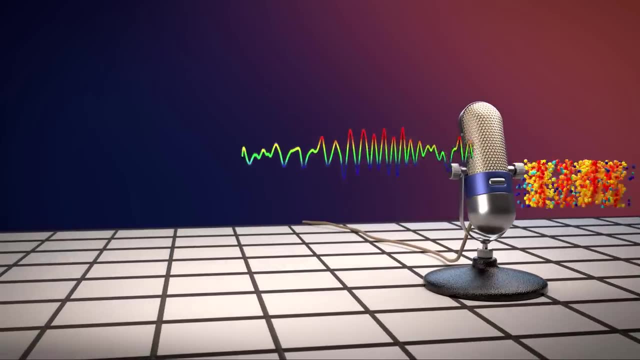 air particles to bounce into one another, thus creating a sound wave. The sound wave propagates throughout the room and hits your eardrum or a microphone, and the waveform looks like this: The difference between the balloon popping and the running faucet is the way the air 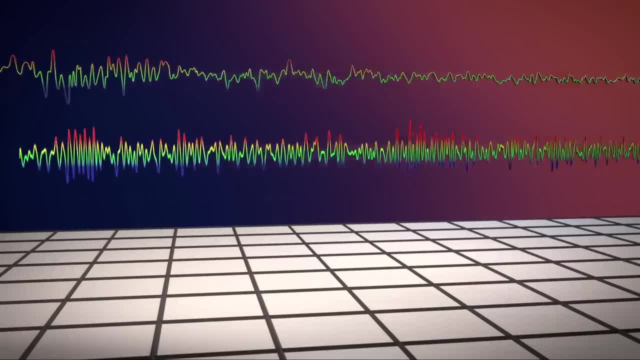 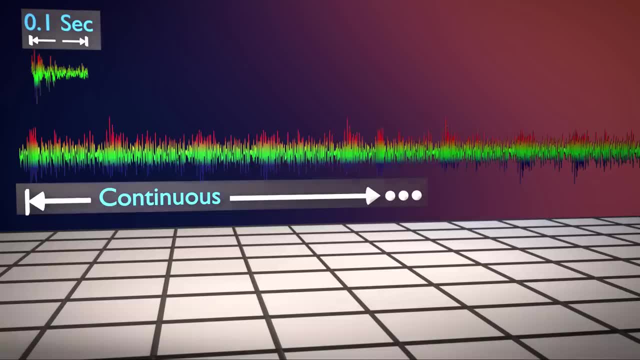 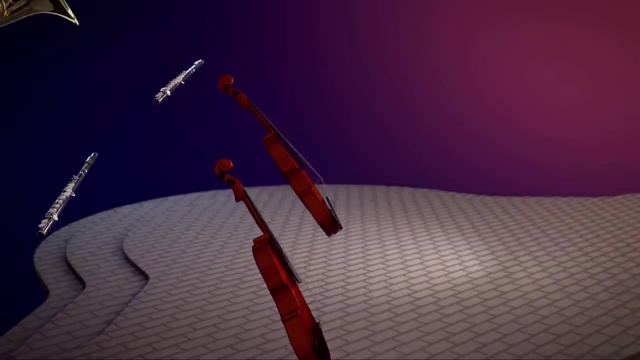 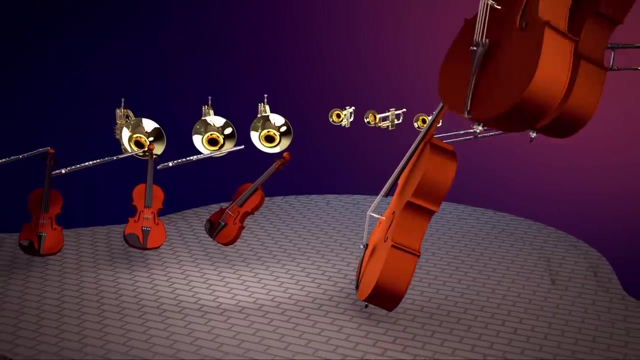 particles are moved, which can be seen in the shape of the waveform. Another difference is that the sound of running water is continuous, whereas the balloon popping only lasted a tenth of a second. Now let's consider a significantly more complex sound. This sound of Beethoven's Ninth is constructed from dozens of instruments. 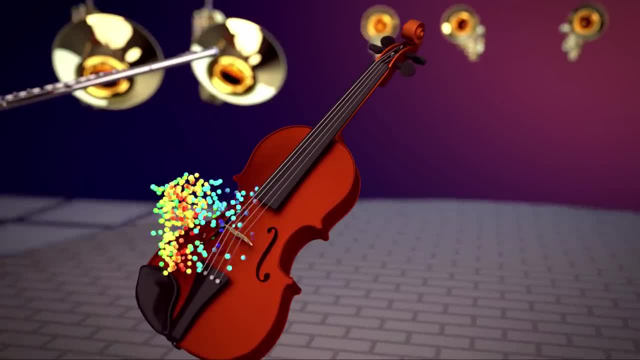 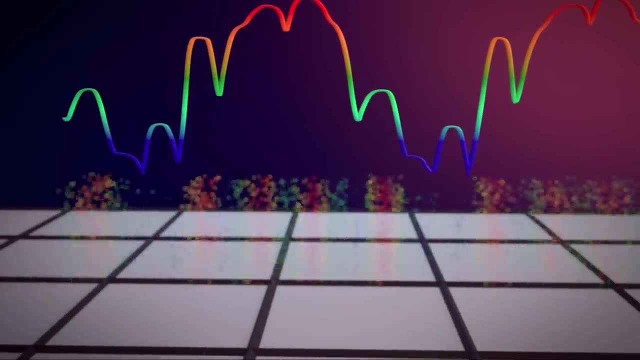 Each instrument, when played, applies a force to the air particles around it, thus causing the air particles to bounce into one another, thereby generating a sound wave. So when the waveforms of different instruments meet in the air, they combine to make a new. 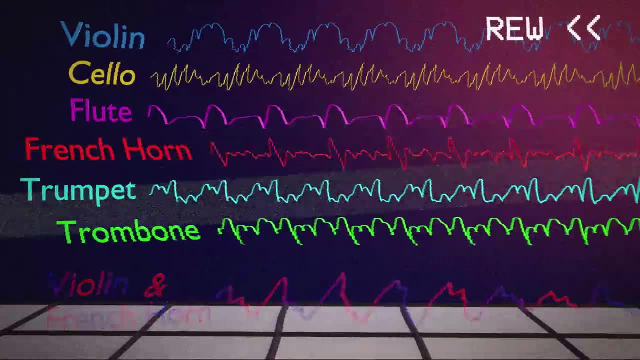 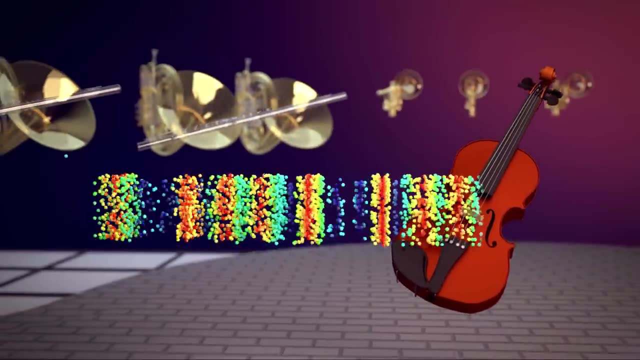 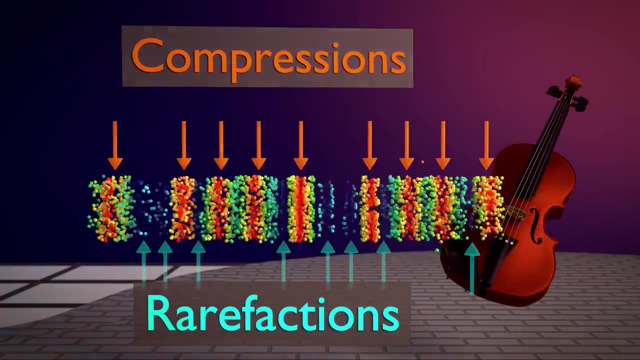 unique waveform or sound. Wait, wait, wait. let's actually rewind and clarify three quick things. First, this animation properly shows how a sound wave is a sequence of alternating compressions and rarefactions. however, it doesn't show how sound propagates in all directions. 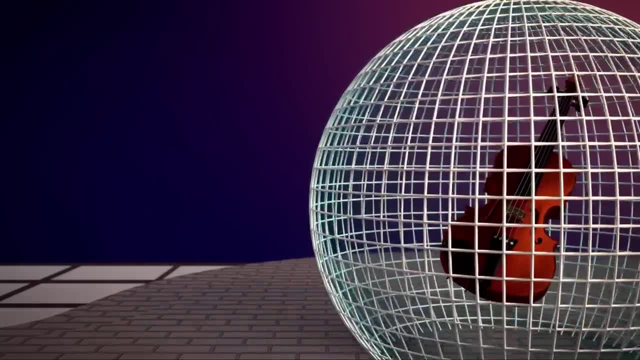 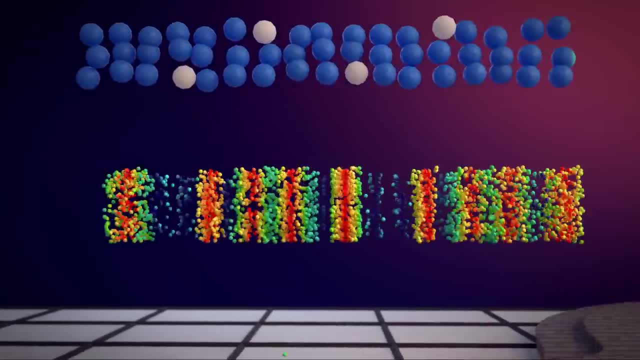 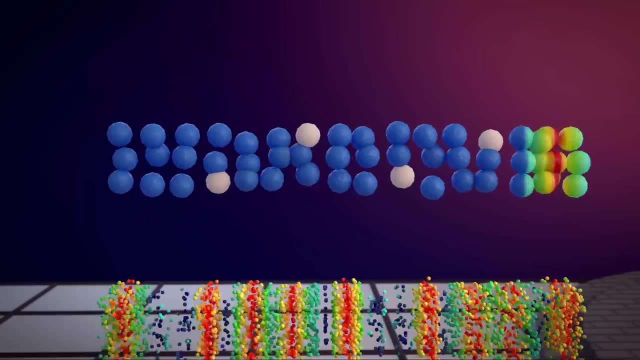 It propagates kinda like this as an expanding sphere, so just keep that in mind Also. second, with this animation it looks like the particles are traveling. however, in reality it is the force of the air particles that is traveling, And this propagation of force, along with the alternating compressions and rarefactions, 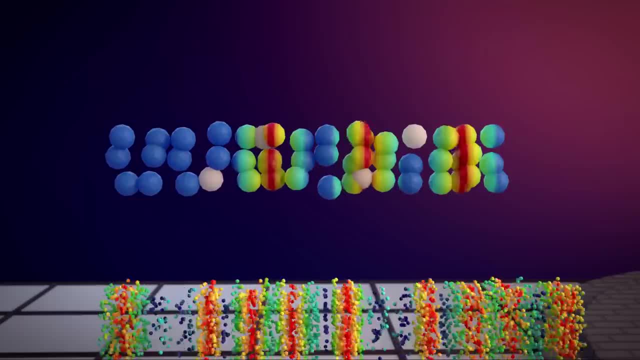 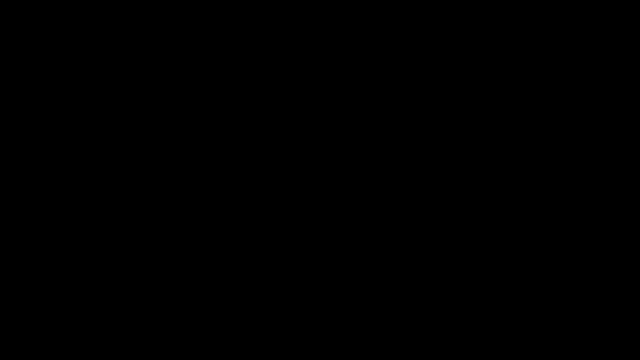 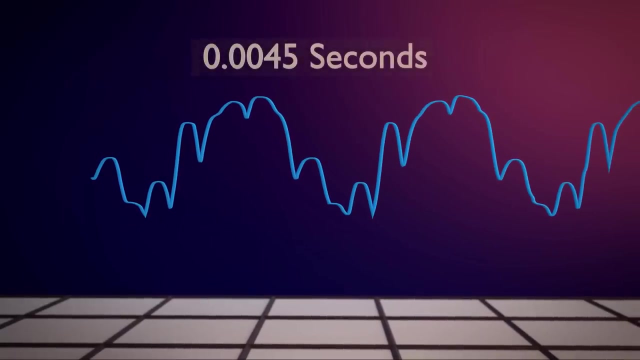 is what constitutes a sound wave. Take a look at the video How Sound Travels to better conceptualize this bouncing-like movement of air particles. And finally, third, this sound waveform is just a quick snapshot of what a sound wave looks like. It's about four thousandths of a second in duration. 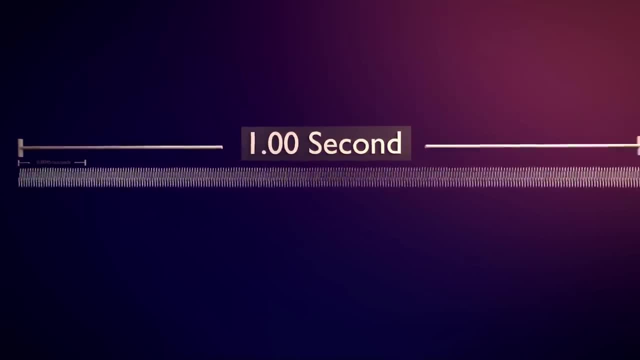 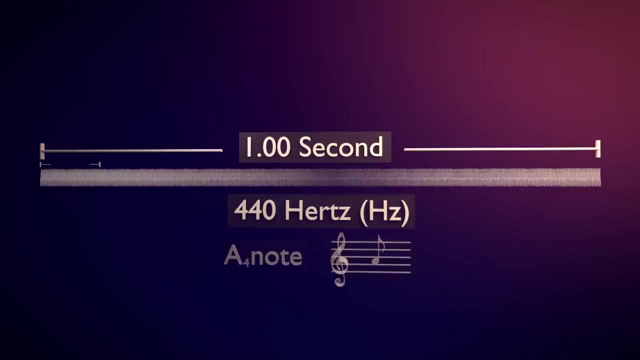 To say it differently, there would be 440 of these waveforms hitting your ear in one second. Or to say it technically, the frequency of this violin sound is 440 hertz. Or to say it musically, it is a musical note A. 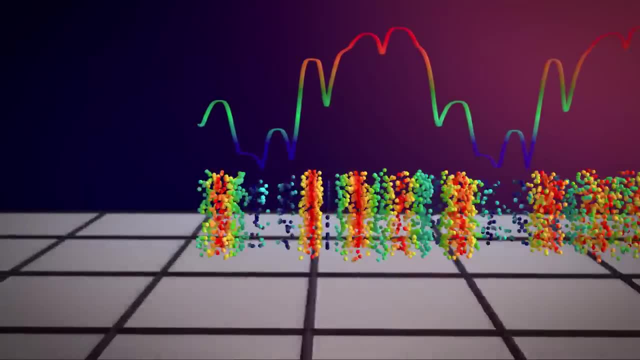 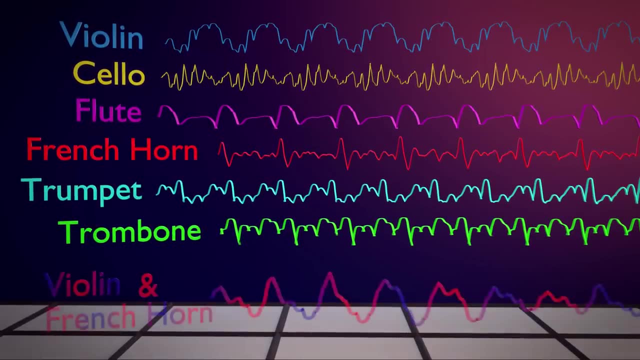 Okay. so now that we have those details clarified, let's jump back to where we were. So when the waveforms of different instruments meet in the air, They combine to make a new, unique waveform or sound. With simple combinations of instruments, our brain is able to analyze this combined waveform. 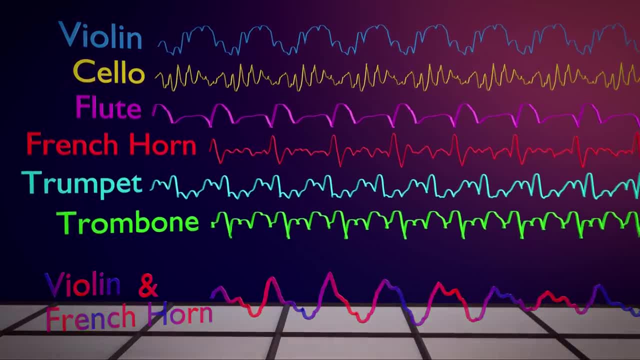 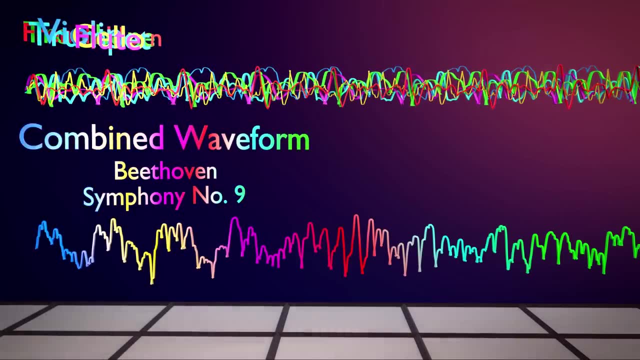 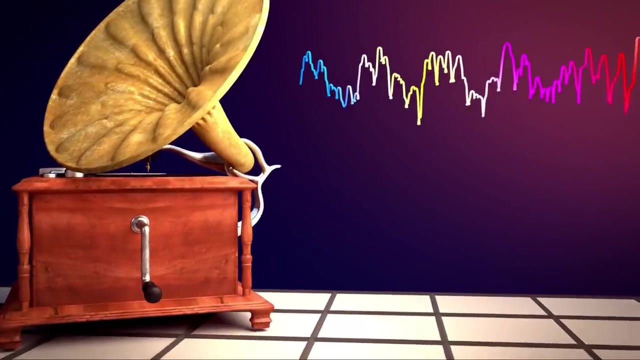 and pick out individual instruments. However, when many instruments are combined, only a trained ear would be able to determine all the instruments used to create the music, because the combined new waveform is so dissimilar to the individual instruments. Furthermore, Furthermore, To record and play back the sound of Beethoven's Ninth Symphony, we would just need to convert the pressure waveform in the concert hall into something like the movement of a needle. 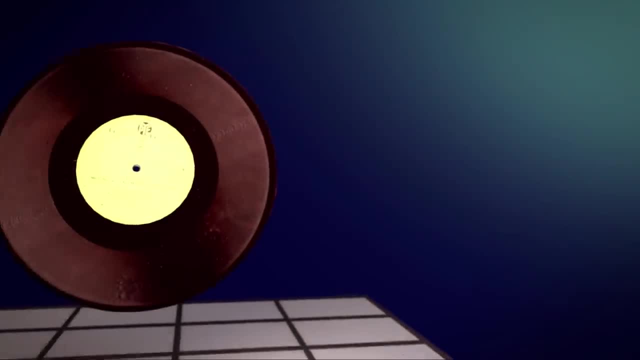 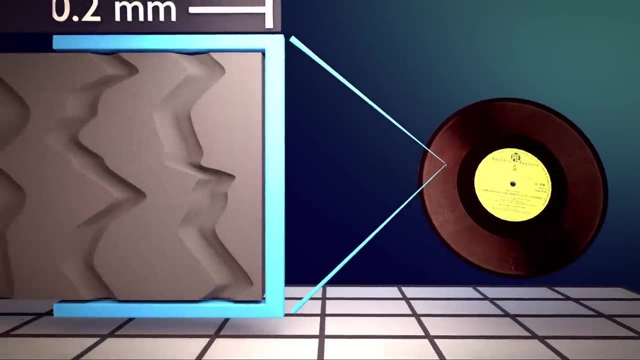 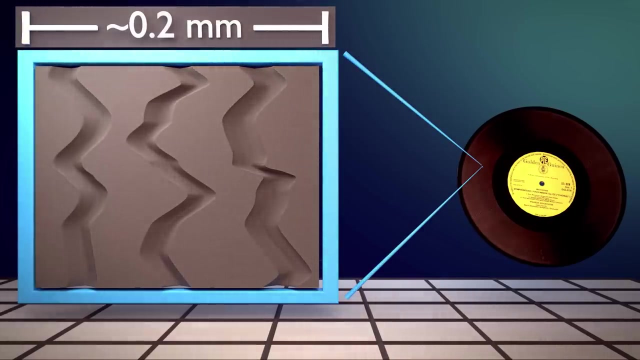 This is the core concept behind vinyl records. A device measures the force or pressure levels from the air particles in a concert hall or recording studio and graphs them into the grooves. on a vinyl record You can see how the shape of the grooves closely resembles the waveforms we have been talking about. 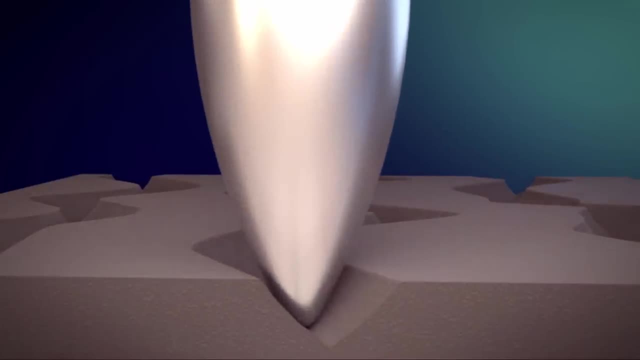 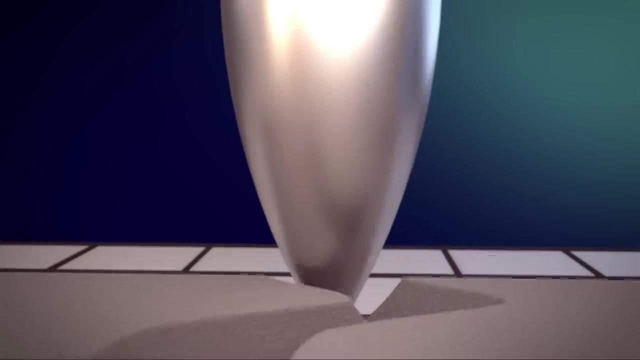 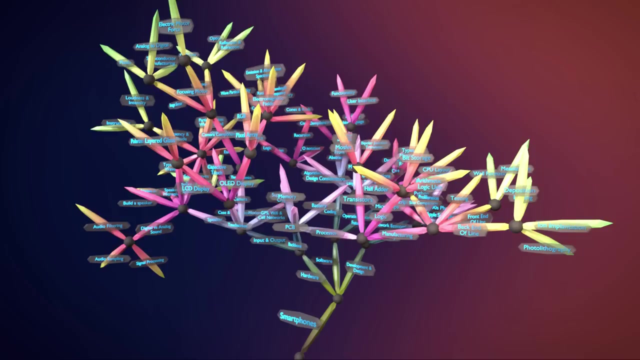 To play this record, a needle just needs to follow the recorded grooves and convert this motion into the motion of a diaphragm, which applies a force to the air particles, thereby reproducing the original sound. Thanks for joining us in learning about sound. If you have any further questions, post them in the comments below. 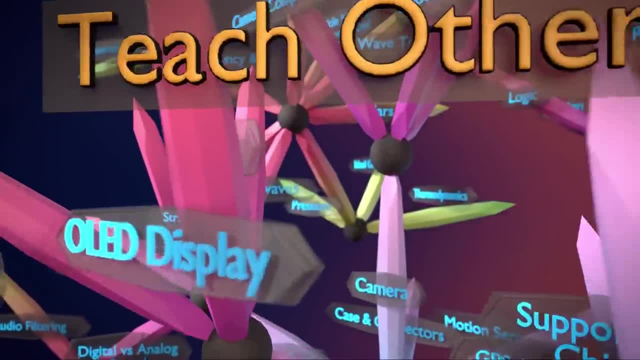 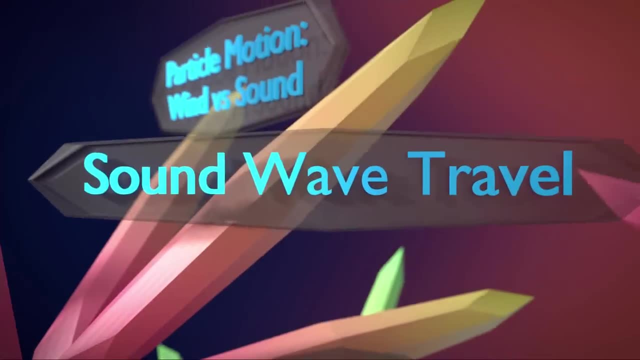 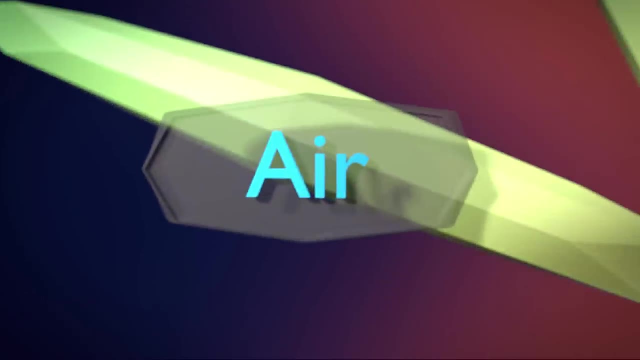 Subscribe, like and tell your friends and family about something you learned. This episode is about understanding what sound waves are. Branches from this episode are: how do sound waves travel, understanding pressure, how ears work, how a microphone and speaker work, understanding air frequency and amplitude, loudness and intensity. and understanding wind movement versus sound. 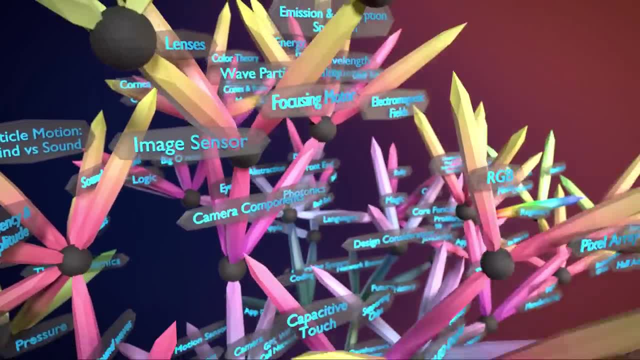 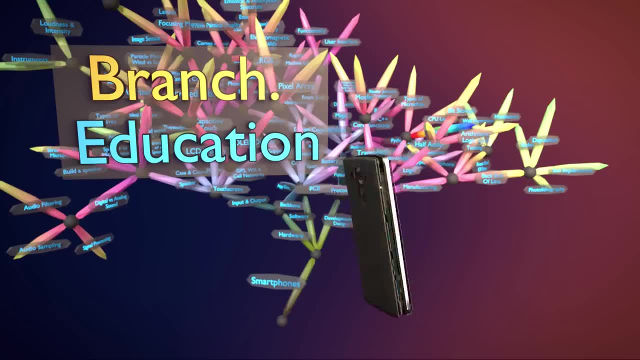 Thanks for watching and until next time. consider the conceptual simplicity, yet structural complexity in the world around us.